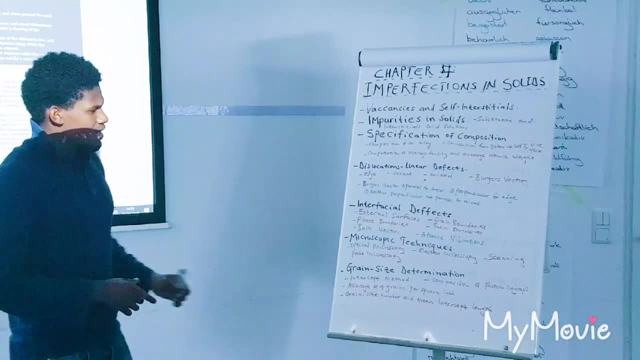 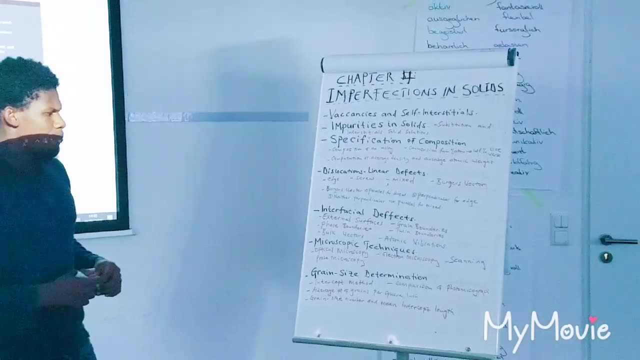 We are going to see that as well, And next we are going to see interfacial defect. We started this in chapter 3.. When we talk about grains, we talk about grain boundaries. It is very, very important from the surface of the material. 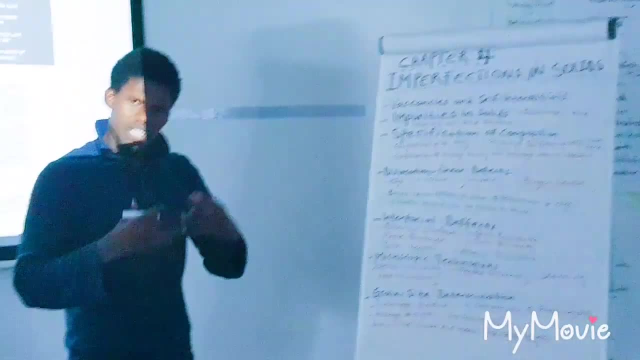 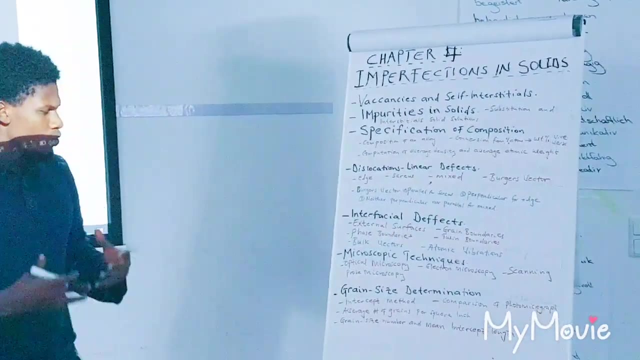 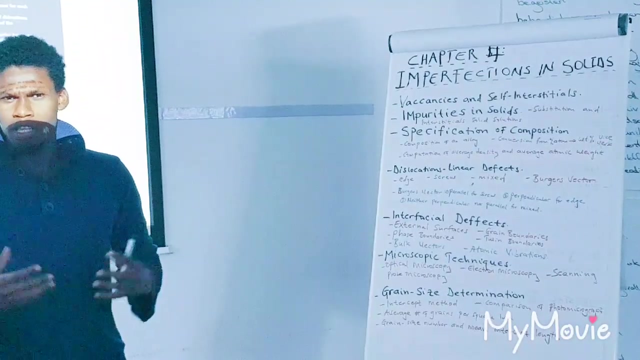 How can you determine the effect or the defect that these materials have, And also the grain boundaries, As well as face boundaries and twin boundaries. So these are the things, Because when you know these things, you are able to manipulate materials. You are able to transform materials to any type that you want. 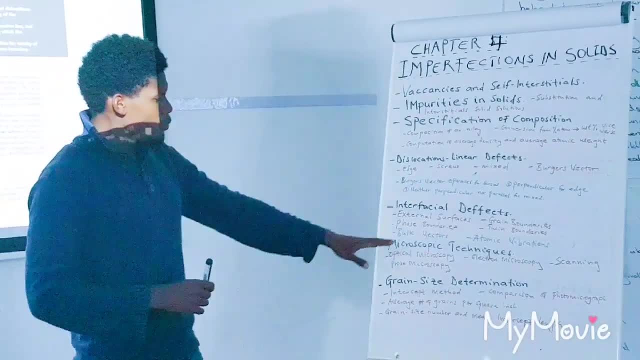 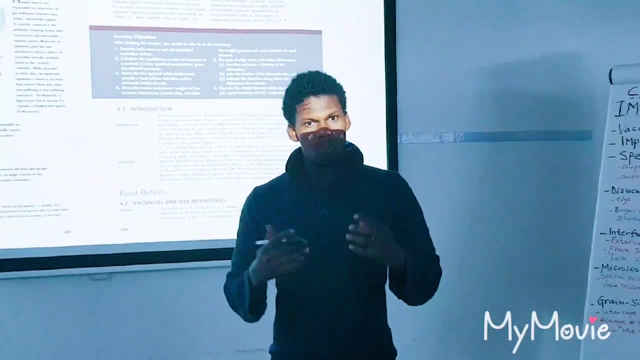 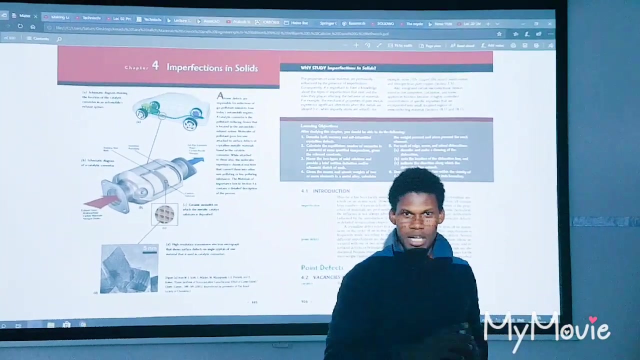 And this is very, very important for you to know that- And we are going to see bulk vectors and atomic vibrations, Because we have been modeling atoms as cycles. But remember, these atoms are vibrating, They are vibrating And it goes back to chapter 1 when we talk about atomic bonding. 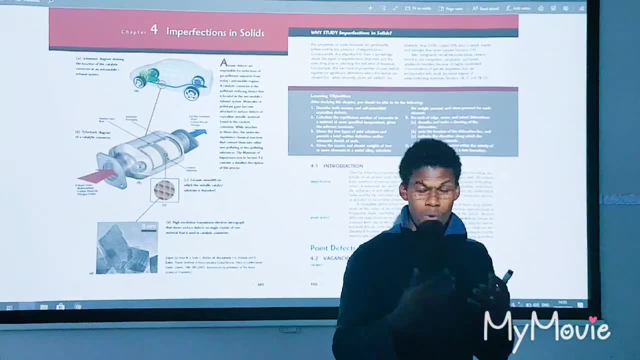 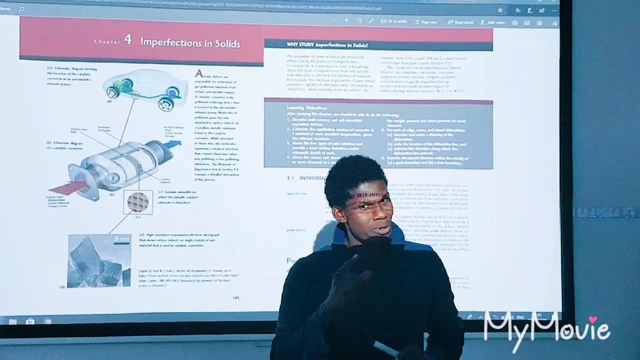 These atoms are not stable. They are vibrating And this is the vibration that we are working with, To know the temperature. So temperature is just like atomic vibrations. So if you know thermodynamics a little bit Or you have the understanding of thermodynamics, 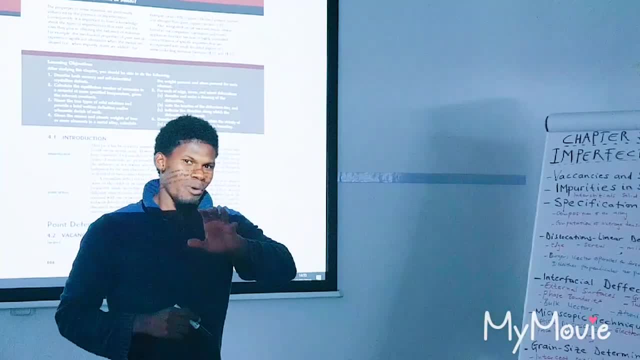 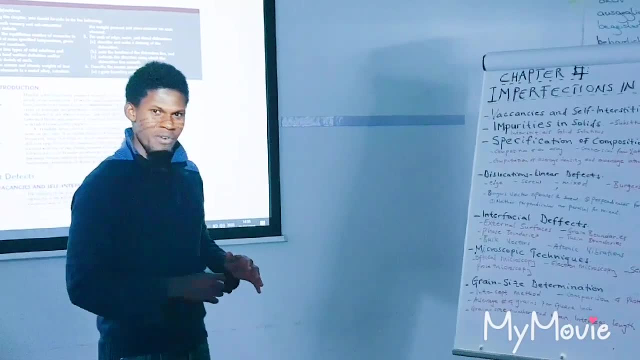 This will help you greatly, But if you don't, don't worry, We are going to demystify it. That is why we have this course. It is to help you to understand the basics, Right from the foundation, of material science and engineering. 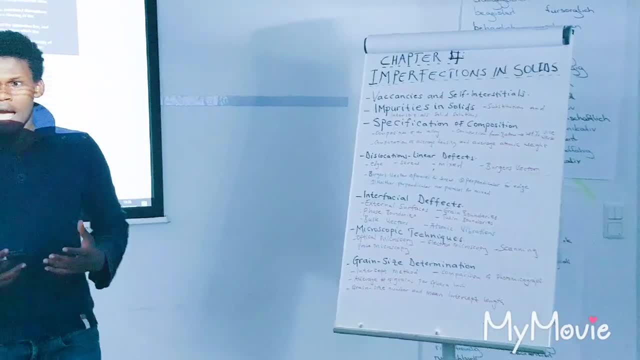 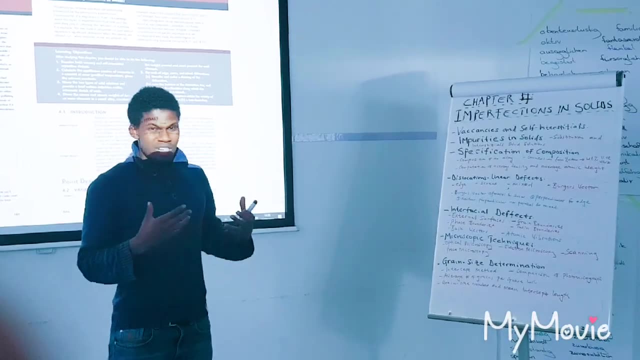 And we are going to talk about microelectronics. This is a microscopic technique, Because if we can talk about these things all day, If you cannot see them, If you cannot feel them, Then it is very, very difficult for you to grasp these ideas or these informations. 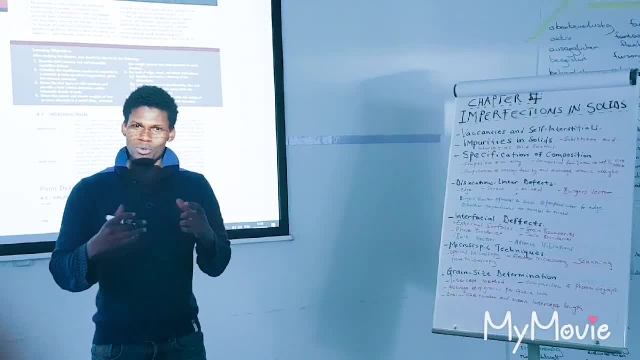 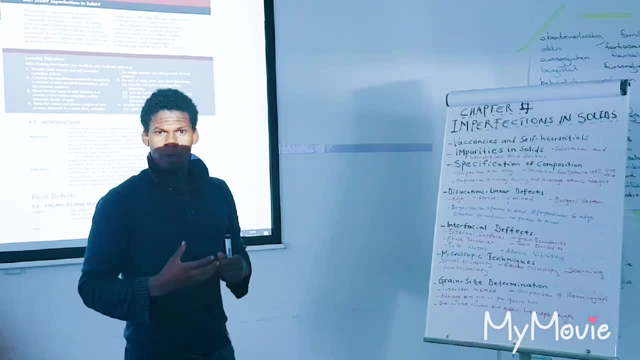 But then we are going to talk about it from the microscopic level: How we can use microscopes to be able to see grain structures. We talk about atoms, We talk about electrons and protons, But we need microscopes. And next we are going to see grain size determination. 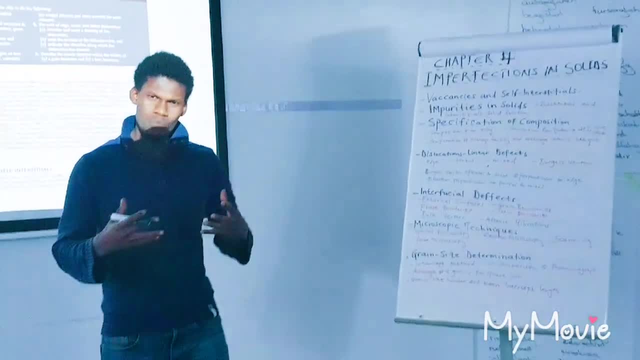 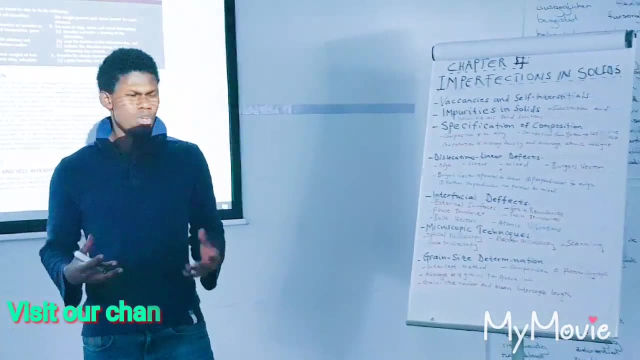 How we can determine these grains. That is why we have methods that we come up with In order for us to be able to determine these grains And the average and the grain size number. Why at all? So this is basically chapter 4.. Imperfections in soil.